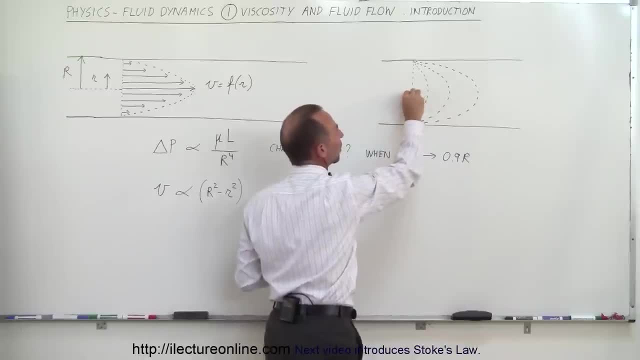 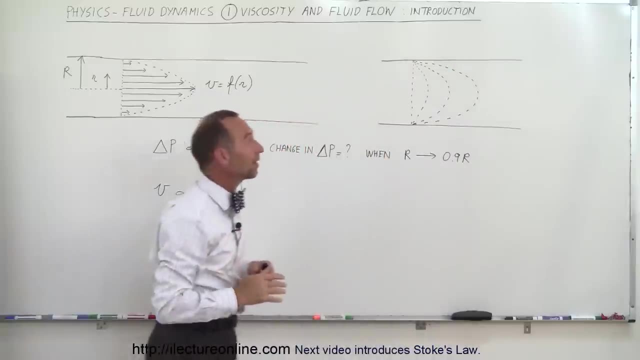 faster. the ones away from the middle travel slower. you can see that these molecules end up over here, while these molecules will end up over there, and those molecules will not travel very far in the same amount of time. and that's how fluid flows through a pipe because of viscosity. Now, 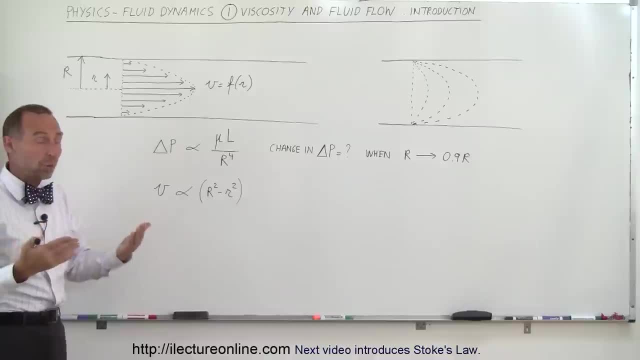 that's very different from what we talked about before, when we talked about Bernoulli's equation. The only time that pressure would change- and with Bernoulli's equation, was if the velocity changed, because the pipe may get narrower, the pipe may get wider, and that is still the case. 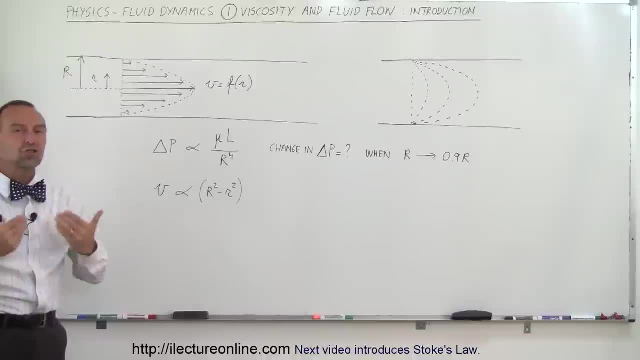 and in the case that the pipe goes up or down, you would expect a change in the pressure. but here what we're indicating is even if the pipe does not change in size, so therefore the velocity remains constant throughout the pipe. and secondly, let's say the pipe doesn't go up. 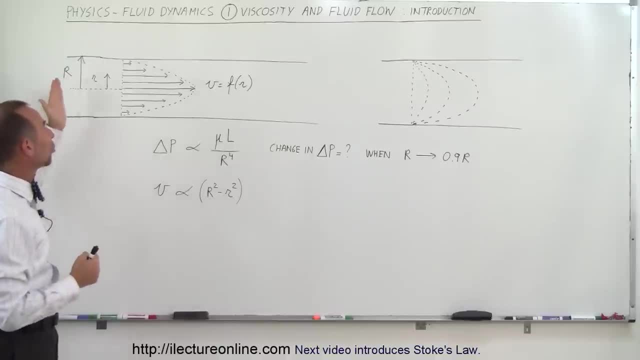 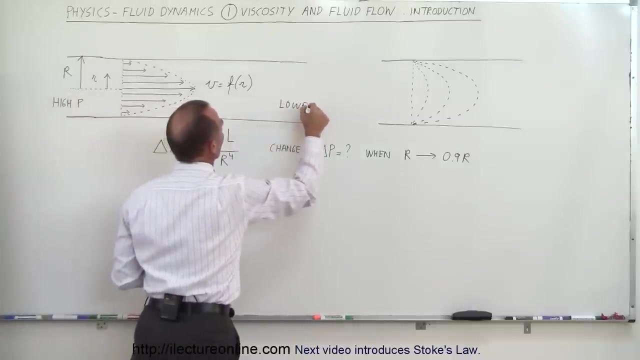 or down, so there's no change in height. we would find that the pressure will change As you travel through the pipe, so we would expect higher pressure here and lower pressure there. so maybe I'll write that down: so high pressure on the left side and lower pressure on the right side. 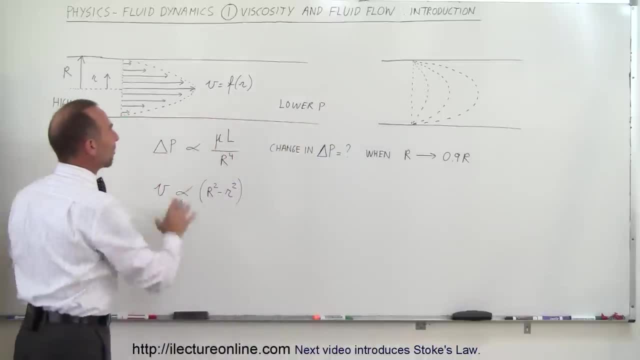 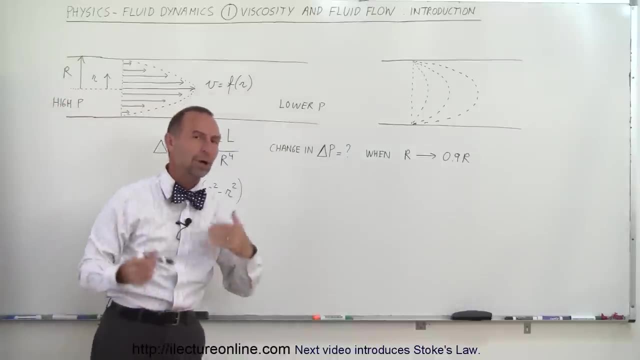 so there's a change in pressure over a certain section of the pipe as fluid flows through the pipe, and so that's where this delta p comes from: the change in the pressure from one point in the pipe to the other point of the pipe due to viscosity. What was discovered was that that 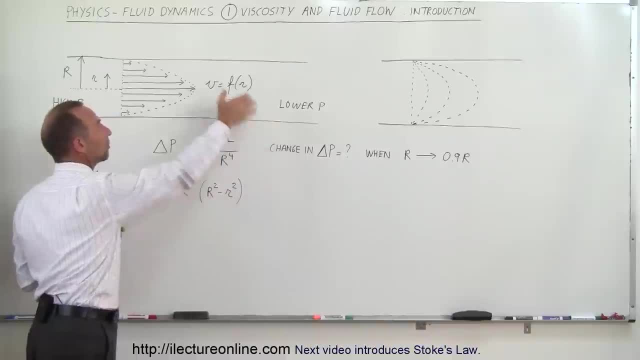 change in the pressure from one point in the pipe to another point in the pipe is. the viscosity here is equal to the coefficient of viscosity times the length of the pipe divided by the radius of the pipe to the fourth power. r is the radius, l is the length of travel. Now, this is only valid if l is not. 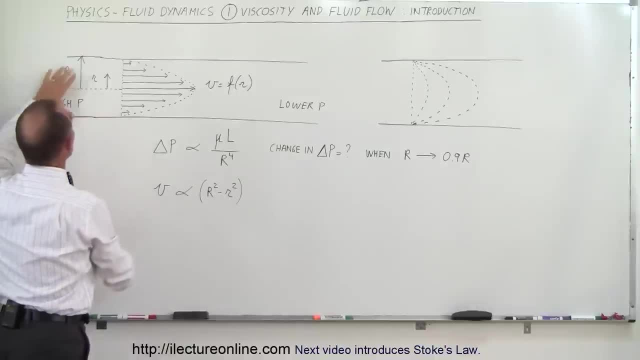 too small, because if the pipe is very short there are some edge effects. as the fluid goes into the pipe- whoa, I'm dropping my pen here from all that excitement about this- and as the fluid leaves the pipe, if the pipe goes up, the velocity changes. so that's the point in the pipe is equal to the 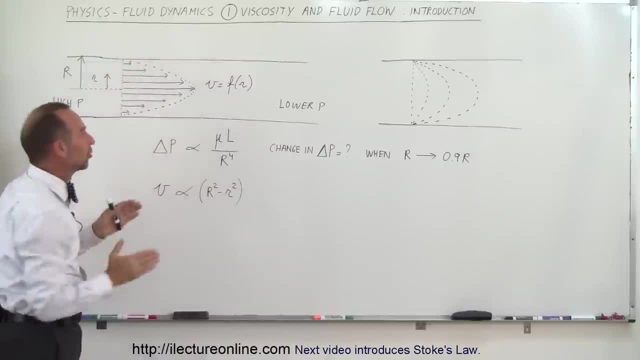 coefficient of viscosity is very short. you have these edge effects, so we cannot take those into account. we want to make sure that the pipe is long enough so we're not deceived by those edge effects. but anyway, the change in the pressure will be equal or not equal, but proportional to that ratio. right there we also. 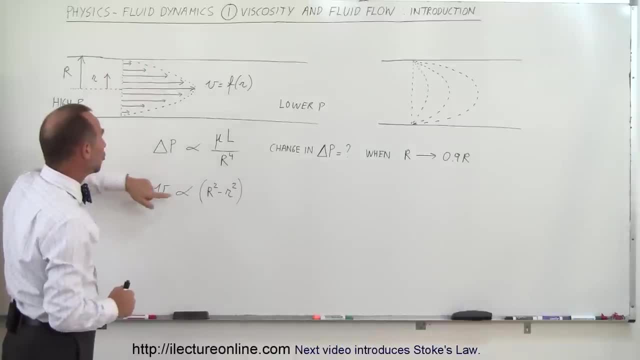 know that the velocity in a pipe like this changes and therefore is proportional to the radius squared of the pipe minus where the point in the pipe you're considering. so let's say, if r is small, r is equal to big r. but other words, how fast are the water molecules or, in this case, any fluid? 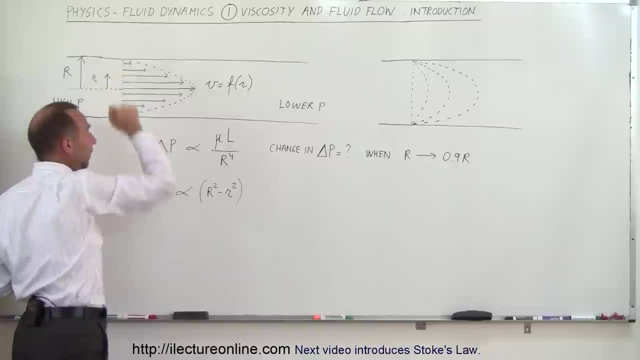 molecules, that's heavy water, any fluid molecules moving along the edge of the pipe. well, if r is the same size as r, it's basically zero. and then you can see that if r is zero, if little r here becomes zero, that would be the maximum velocity. you have, the maximum velocity of fluid in the 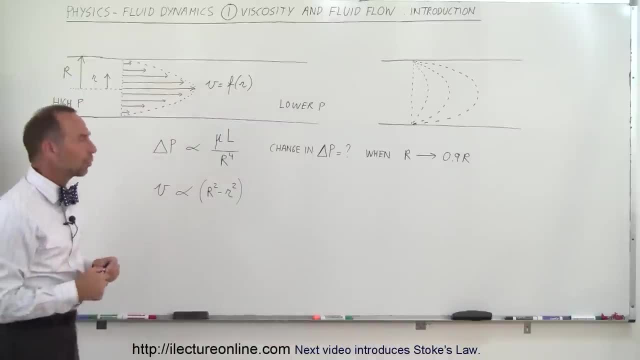 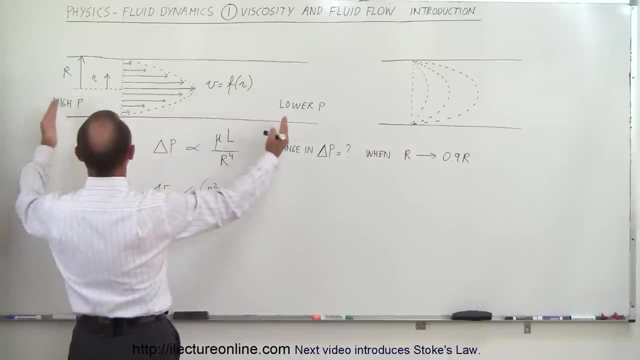 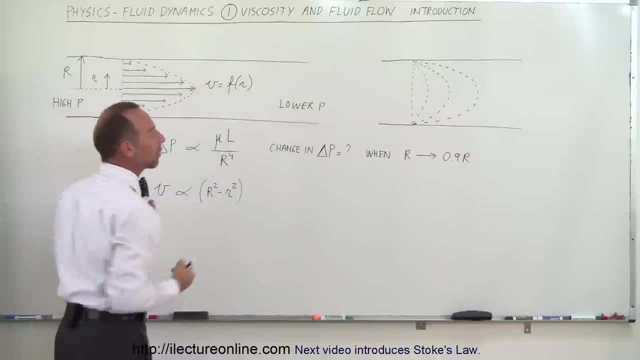 there, there would be a certain pressure drop. well, what would be that pressure drop if the pipe was narrower? well, notice that it's proportional: one over r to the fourth. and so let's say that r now changes to 0.9 r and you're trying to push the same amount of fluid through there. what would 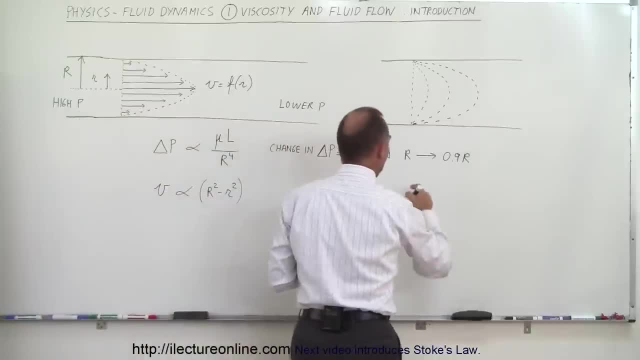 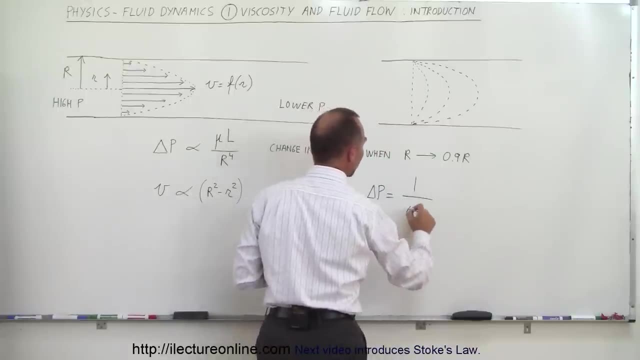 happen. so what's going to happen is that the change in the pressure delta p is going to now be equal to 1 over 0.9 r to the fourth power. i shouldn't say equal, i should say proportional, because we don't have a constant. 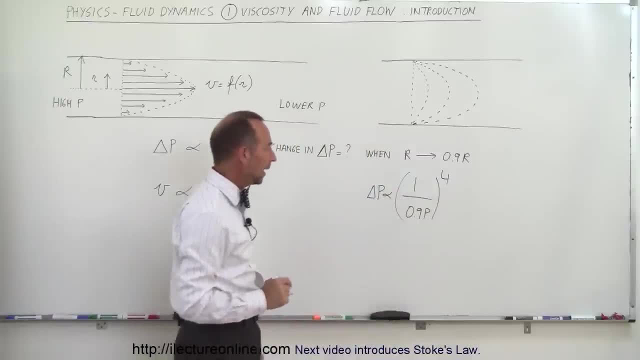 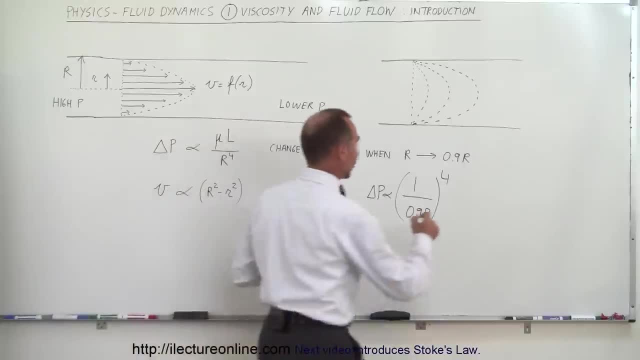 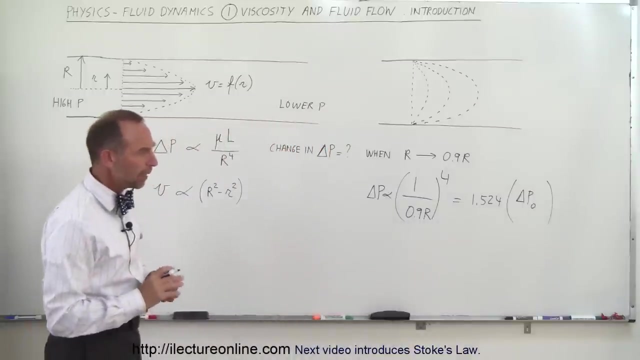 that. notice that it's now 1.524. so this would be equal to 1.524 times what it was originally- the delta p initially, if r was equal to 1r. what that means is this is kind of there's a kind of a.